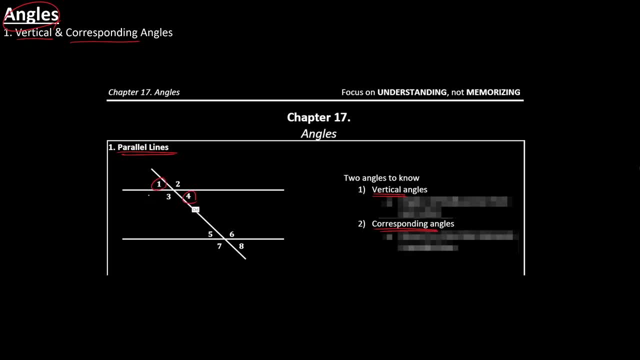 difference between the two Vertical is going to be two angles that are across from each other and they are going to have the exact same measure. So one and four: same measure. right five and eight: same measure. six and seven: same measure And corresponding angles. 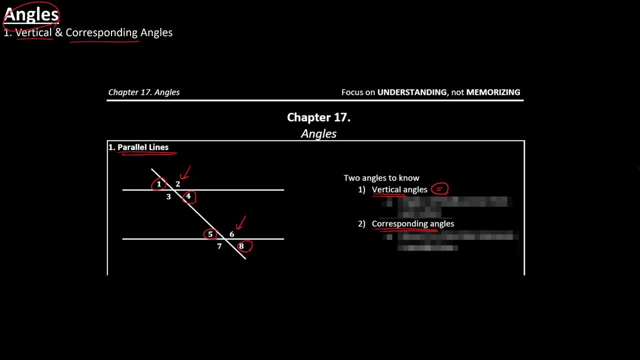 are going to be the angles that are on the same corner, same corner of two different parallel lines. So if you look at angle two, it is on the upper right corner of this line and six is also in the upper right of this line. That means these two angles are going to be the same. 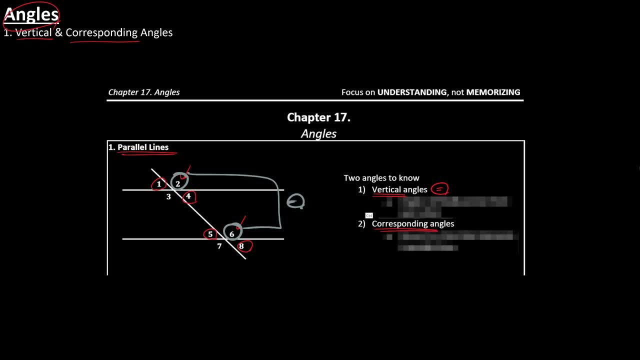 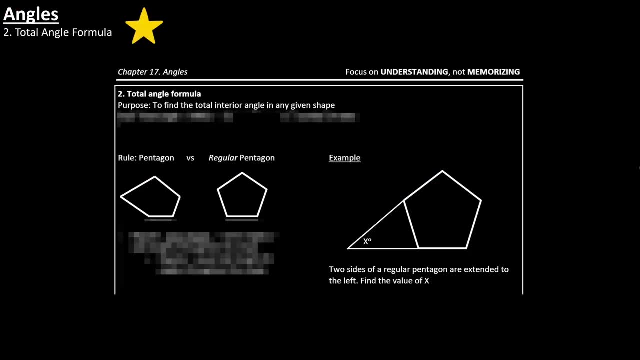 same thing for three and seven, five and one, four and eight. Okay, you want to know two of these angles. Next, you also want to know about the total angle formula, And the purpose of the total angle formula is for you to find the total interior angle in any given shape. So, for instance, when you 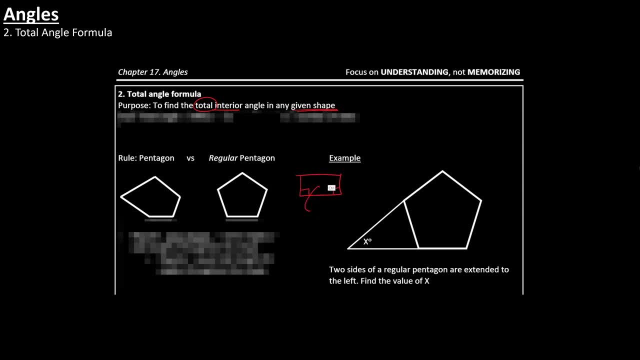 have a rectangle, we know that the angles all add up to 360, right, Because total interior angle angles on the inside. So angles on the inside they all add up to 360.. But what about a pentagon When you have five sides? what is the sum of all the angles on the inside? What if you have a? 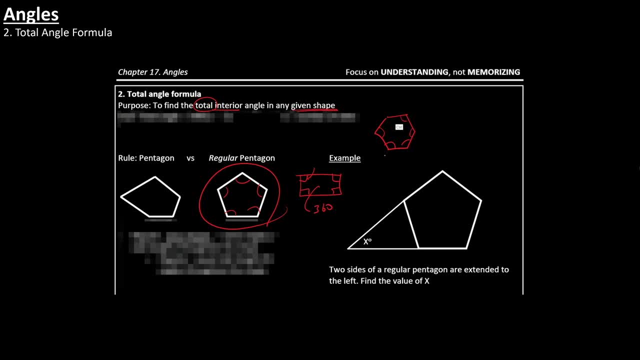 hexagon: What's the sum of all the interior angles? You want to know how to find it so you can answer a question like this, And this is something you will see on the SAT. It's actually the exact question you will see on the SAT. Next, you also want to know what the exterior angle theorem is. 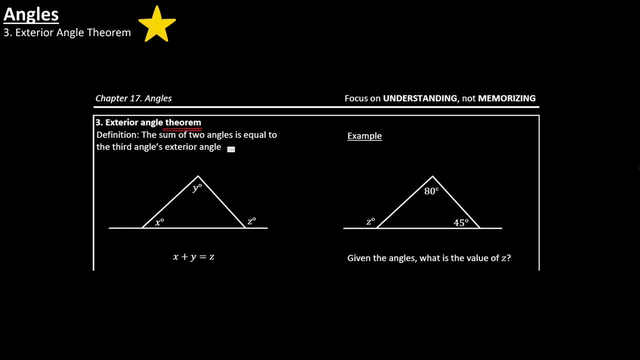 And what the theorem tells you is that the sum of the two angles is equal to the third angle's exterior angle. That seems like a mouthful and it's pretty confusing, So let me explain. When you have a triangle like this right, There are three angles: first angle, second angle. 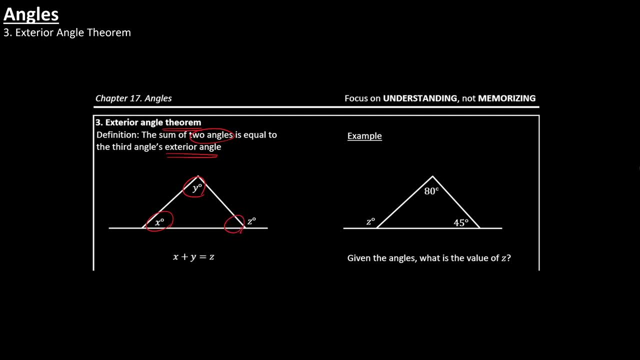 and the third angle, And what the exterior angle theorem tells us is that the sum of two angles, right, So the sum of two angles- is equal to the third angle's exterior angle, meaning exterior, meaning outside. So third angle's outside angle, right there, Does that make. 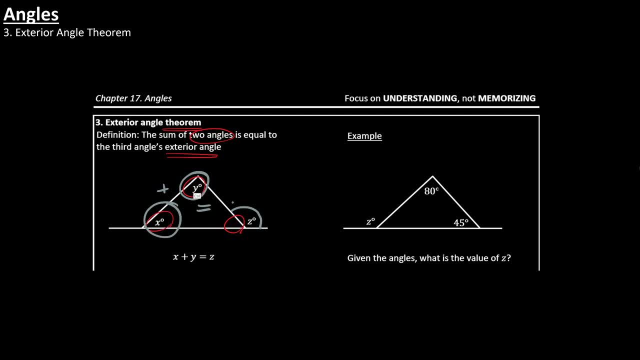 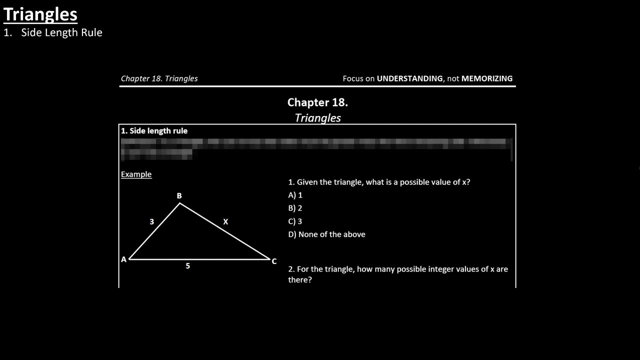 sense. So X plus Y, their measure is equal to the third angle's exterior angle, which is Z, right there. So formula looks something like that And if you understand it, you should be able to solve this example to the right. Make sense, Cool. Let's move on to triangle. The first triangle is going: 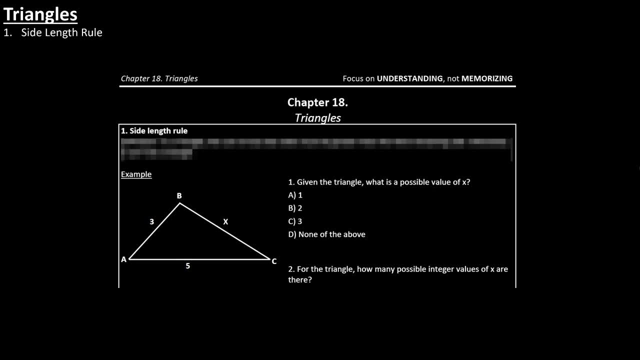 to be a very big chapter because it's very it's tested a lot on the SAT And there will be a lot of things for you need to know. but the first thing you need to know is going to be the side length rule And, if you want to, if you understand what side length rule is. 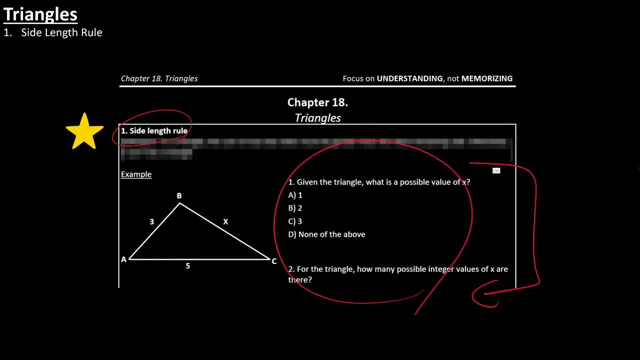 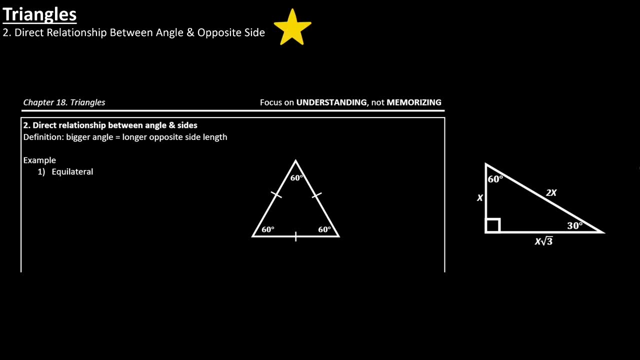 then you should be able to solve these questions, And they are the exact questions that you will see on the SAT as well. Next, you also want to know that, within a triangle, there is a direct relationship between angle and the opposite side. So what do I mean by that? Well, let's think about. 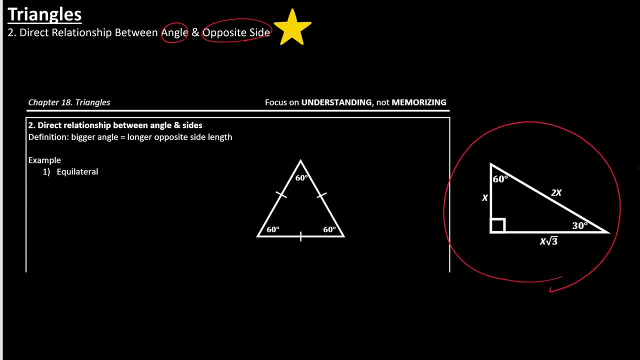 a special right triangle: 30,, 60, 90 triangle. We know that within this triangle there is a relationship: The side is the opposite side. So what does that mean? Well, let's think about a that's opposite from 30 is going to be X and side opposite from 90 is going to be 2X. right, But why? 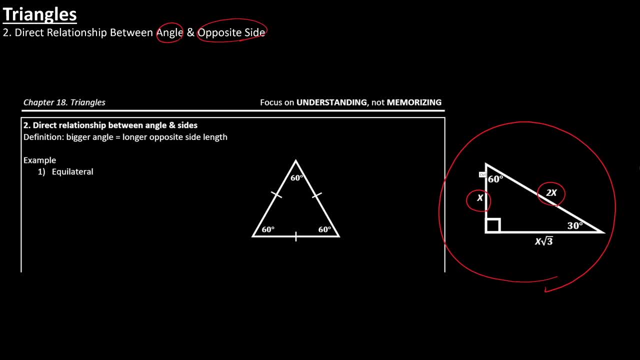 is that the case? Why is this length bigger than this length right there? Well, that's because there is a direct relationship between angle and the opposite side. Direct relationship meaning: as angle gets bigger, the side length will also get longer, And as one gets smaller, the other one. 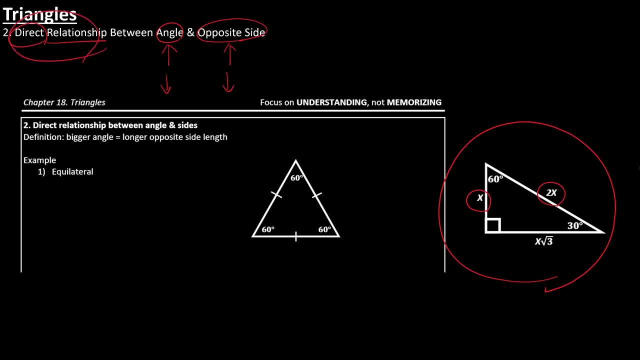 gets smaller. That's what direct relationship means. So, within this special right triangle, the reason why the side opposite of angle 30 is smaller is because it's opposite from a smaller angle. 2X is opposite from 90, which is going to be a bigger angle than 30 degrees right. So direct relationship between: 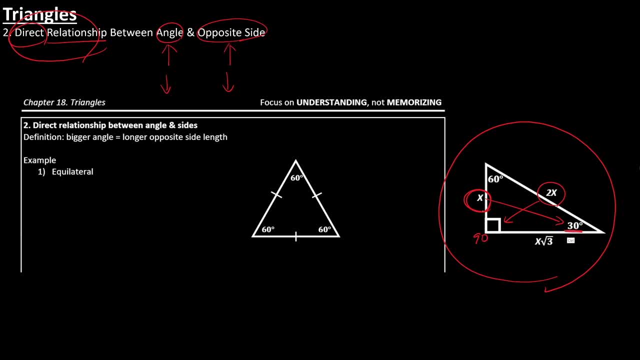 angle and opposite side. This is smaller because it's opposite from a smaller angle And this side is longer because it's opposite from 90 degrees. Guys, make sure you really understand this, because it's one of those things that are not covered in these SAT books And it's really important for you. 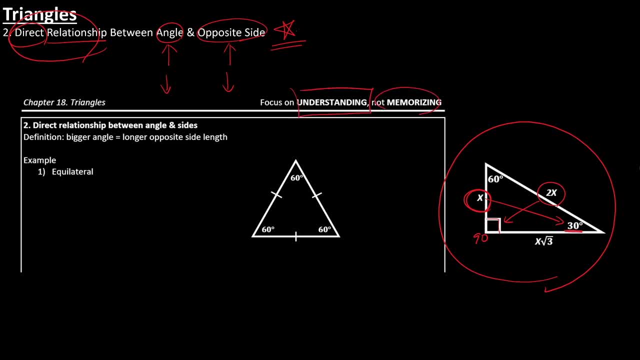 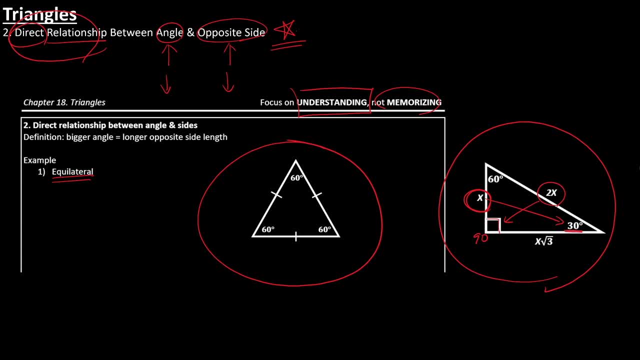 the equilateral triangle- equilateral triangle- you can understand why all the side lengths are going to be the same and why their angle measures are also going to be the same. If you understand it, leave it in the comment section down below. I'll check it for you. Next, you also want to. 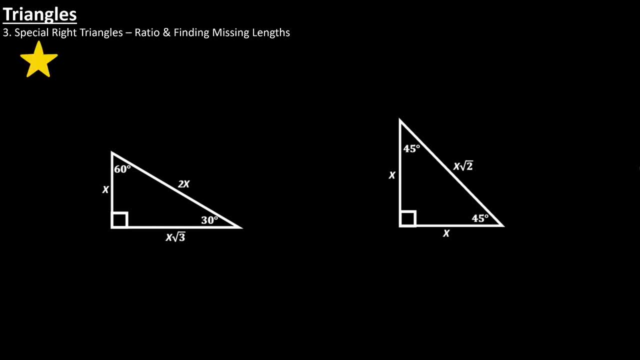 know special right triangles. So there are two types of triangles you need to know. First, one's going to be 30,, 60, 90 triangle. Second, one's going to be 45,, 45,, 90 triangle. You want to. 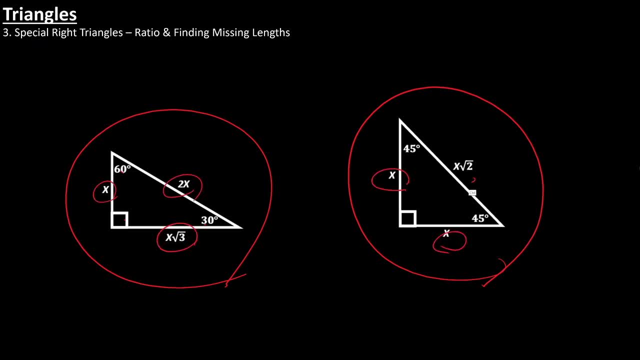 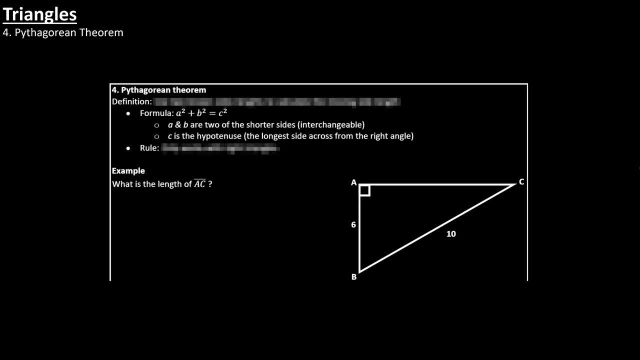 to know how to calculate it. Okay, Next, you also want to know Pythagorean theorem. You want to know what the formula is, how to use it and when to use Pythagorean theorem. So, if you know how to use, 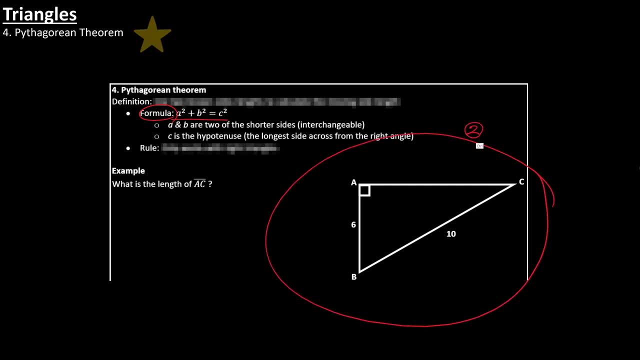 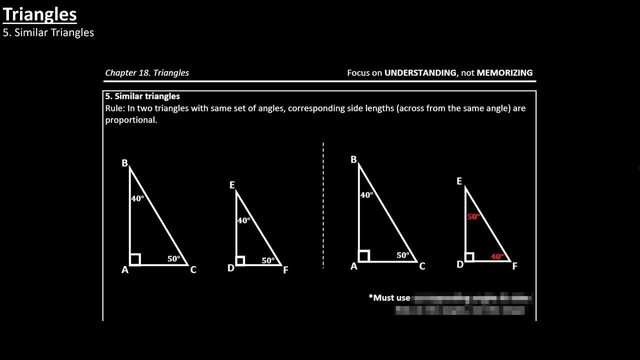 it, you should be able to answer this question. This is like a difficulty two question, but if you understand when and how to use it, you should be able to answer difficulty four or five hard questions. Next, you also want to know what similar triangle is. See the definition of similar triangles is. 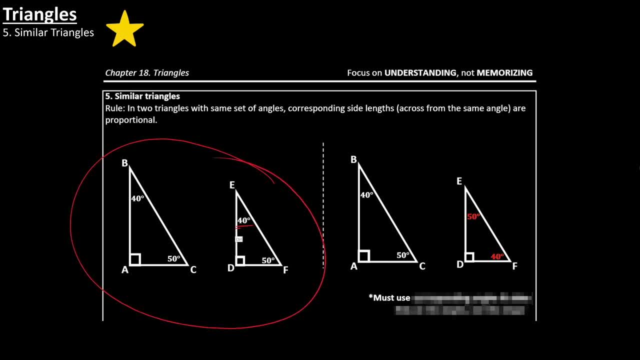 that when you have two triangles that have same measure of angles, when they have same set of angles, then you know that their side length are going to be proportional. Okay, So how the SAT is going to test you on this is that they're going to give you maybe like four, five, six, and give 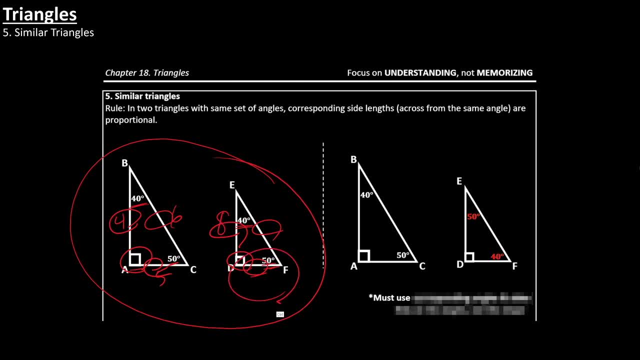 you something like eight. Then you want to be able to know how to solve for this length and this length. Okay, So that's what similar triangle is. You want to know how to find missing side length. Next, you also want to know how to convert radians into angles and angles back into radians. So 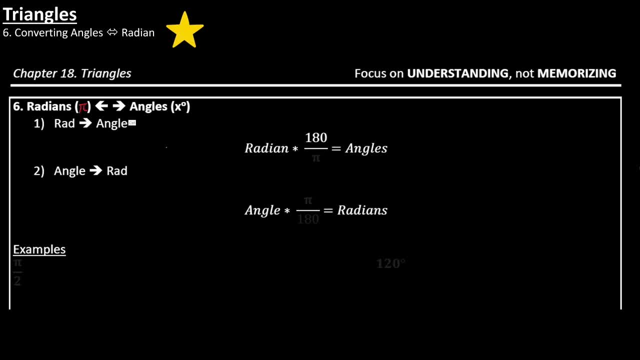 what is a radian? Well, radian is going to be the measure of the angle in terms of pi. Okay. So radian shows you what the angle is using the pi. So whenever you see something like pi over two, that's going to be a radian because it has a pi in it. And when you see something like 120 degrees, 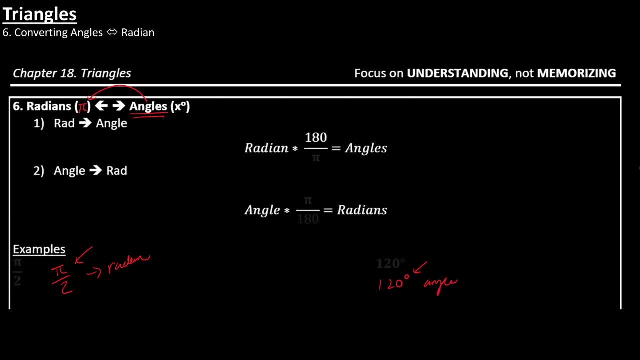 it's going to be a radian. So when you see something like 120 degrees, it's going to be a pi. So when you see something like 120 degrees, it's going to be an angle, because you see the degree mark right. 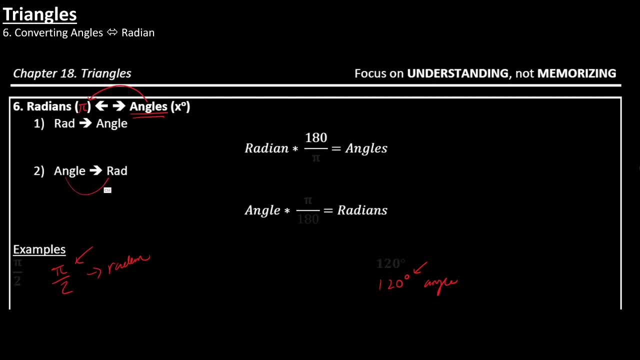 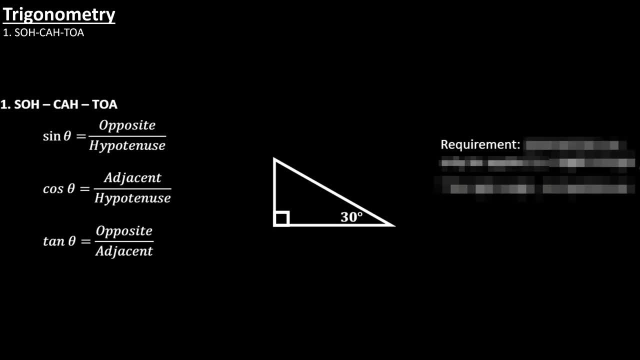 there And you want to know how to convert from angles to radians and radians back to angle, And how you do that is by using this formula, right there. Okay, Let's go to the next chapter, which is going to be trigonometry. So, when it comes to trigonometry, the first thing you want to know 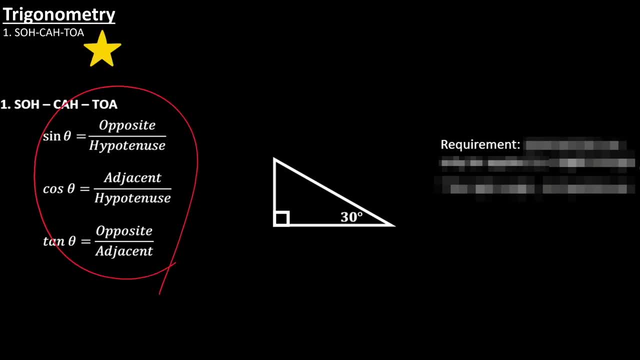 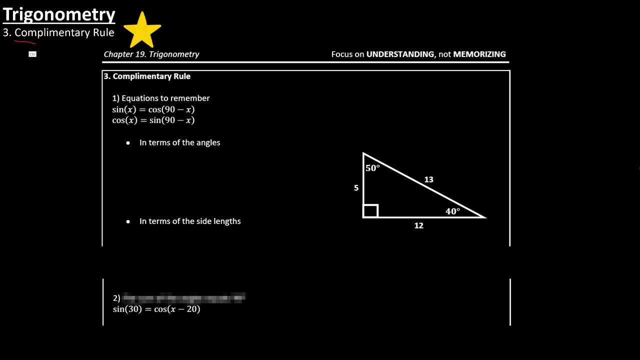 the main thing you want to know is going to be SOHCAHTOA: how it works and how you can use it to find the missing side length, and when to use SOHCAHTOA. And the next thing you want to know about trigonometry is going to be complementary rule. So it's one of those things that are not 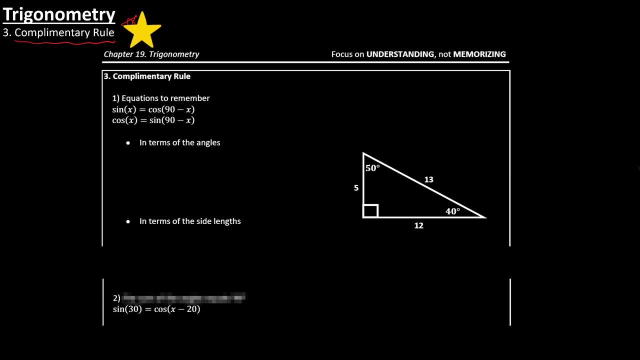 really covered too much in detail, or it's not covered at all on these SAT Amazon books, right, But you really want to know it. It's either you know it or you don't, And by knowing these two things alone you'll be able to answer more questions. So let's go over what they are. 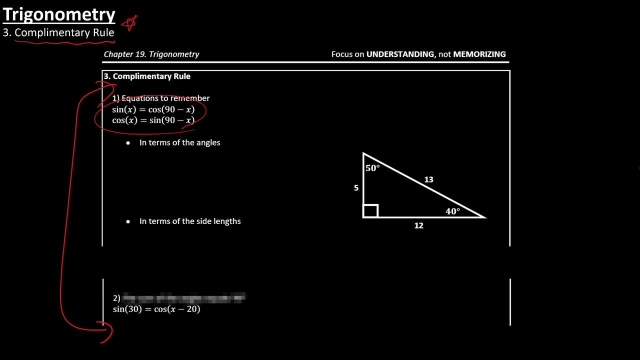 When it comes to complementary rule, you want to know these two equations And these two equations, you want to understand them, not just memorize them, but understand them in terms of angles and side length, Okay. And second, when they give you something like this, this is going to be a 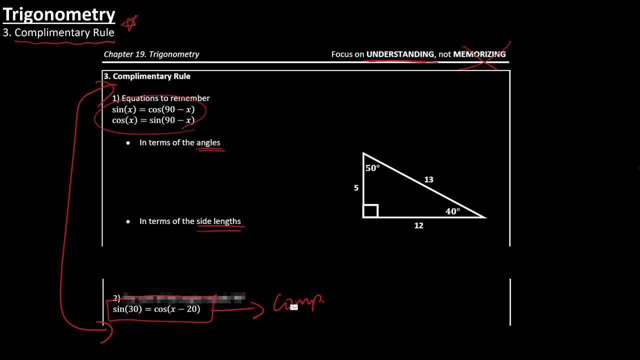 SOHCAHTOA. So when you see something like this, this is going to be a SOHCAHTOA, And when you see SOHCAHTOA, not SOHCAHTOA- complementary rule question- and you want to be able to find out? 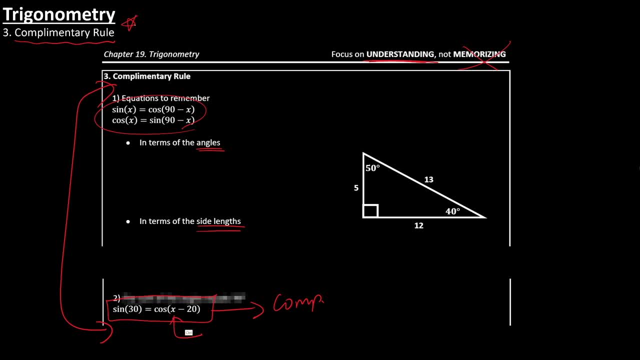 what the value of X is, See SAT will test you on this. You're going to see this exact same question. Okay, That's what the course is designed on: how the SAT actually test you on. Next, that's it for. 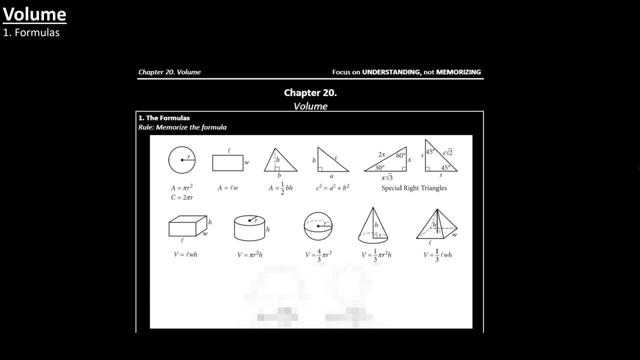 trigonometry. But when it comes to volume, the main thing is for you to memorize these formulas right? So all of these formulas are on the first page of the SAT, section three and section four, And just because they are on the first page, many people just say I don't need to know. 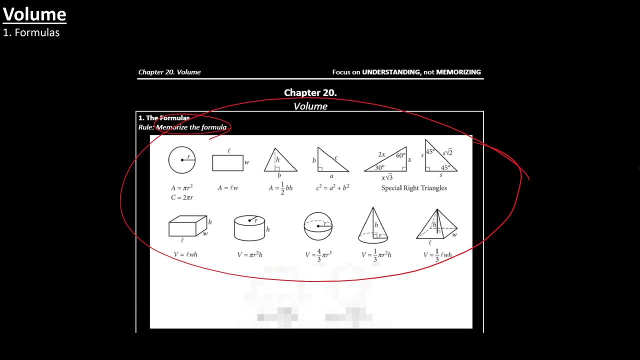 they are on the first page. no need for memorizing. But here's the thing: You will need to memorize these equations, Otherwise you won't be able to solve questions that use these formulas. Like, if you don't have these formulas in your head, then you won't be able to even 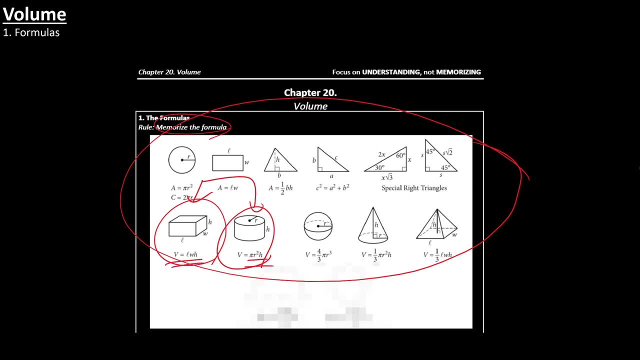 recognize that you're being tested on these formulas. It's one of those things that won't make sense now, but it's going to be one of those things that will make more sense as you take more practice exams and you will thank me for it later. So you want to know those formulas. There are a. 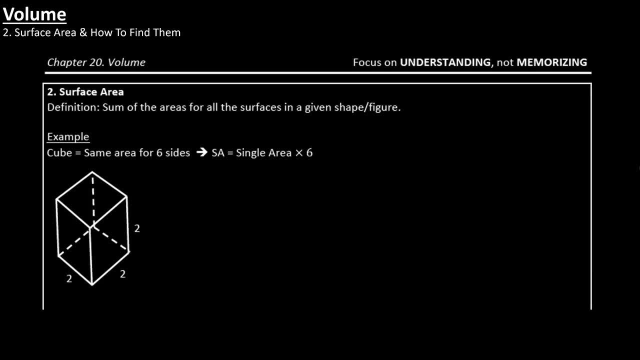 couple more formulas that you need to know, but this is a good place to get started. Next, when it comes to volume, you want to know what surface area is right. You want to know the definition of surface area and how to find the surface area of any given shape or figure. So if 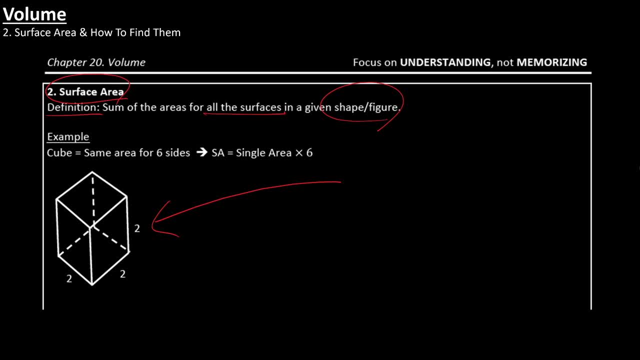 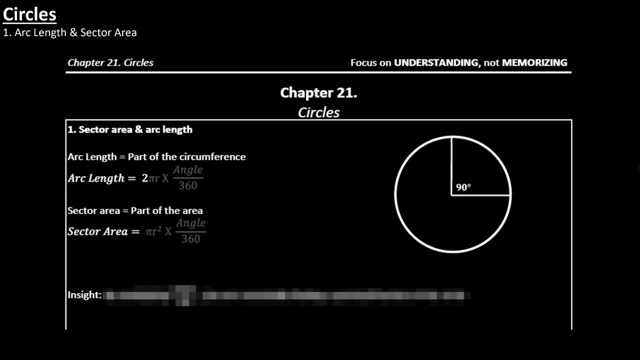 you know how to do it. you should be able to find the surface area of this cube right here, And the correct answer is going to be 24.. Okay, Next let's go to circles. So circle is going to be the second biggest geometry chapter on the SAT. First, the biggest chapter is going to be triangles, Circles. 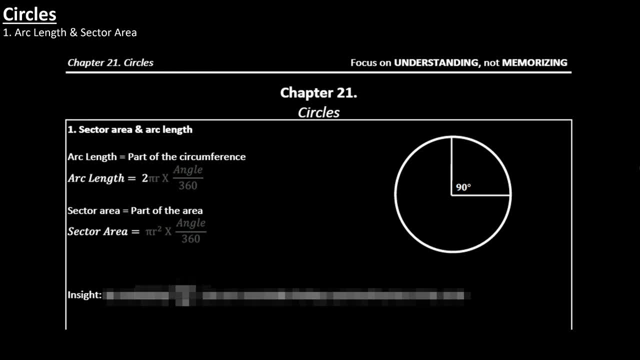 is the second biggest and a lot of things, but we'll break them down. First thing you need to know about circles is going to be arc length and the sector area. Arc length and sector area are just referring to a portion of a circle, Okay, So if you're finding area of this, 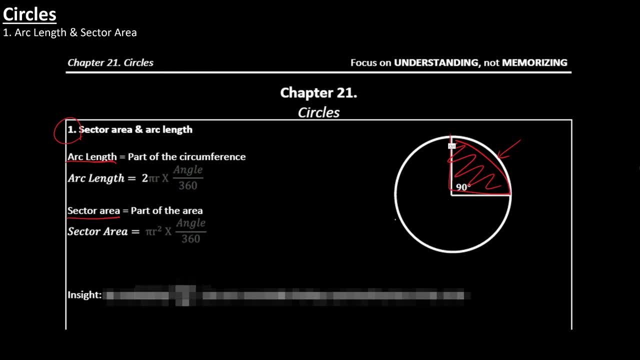 portion right there is known as the sector area. And if you're finding just this length from here to here, from the whole circumference, that's known as the arc length, And you want to know how to find these things. Next, you want to know the difference between central and inscribed angle. 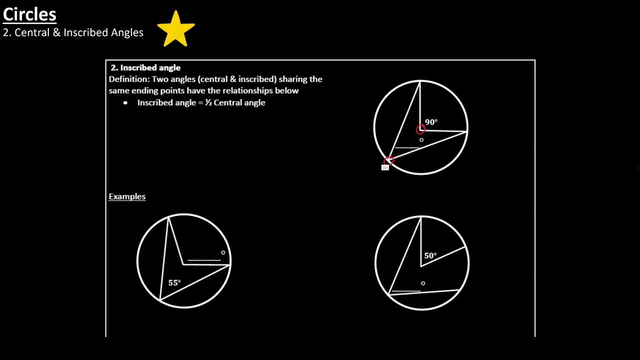 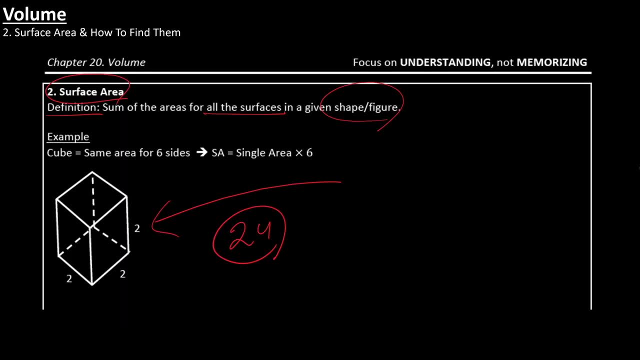 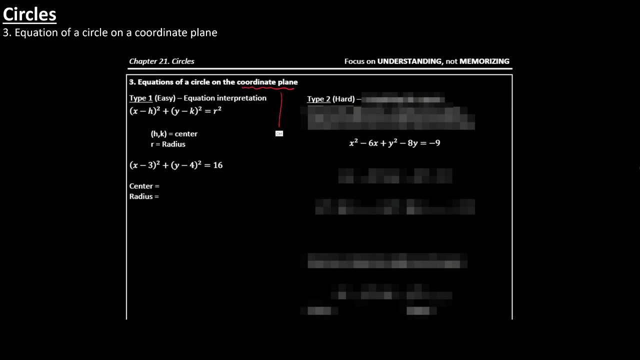 Right there, inscribed angle, right there. You want to know the relationship between these two things, Okay, Next, when it comes to a circle, you might see circles on just as a shape, like so, but SAT will also test you about a circle on a coordinate plane, and coordinate plane is referring to the 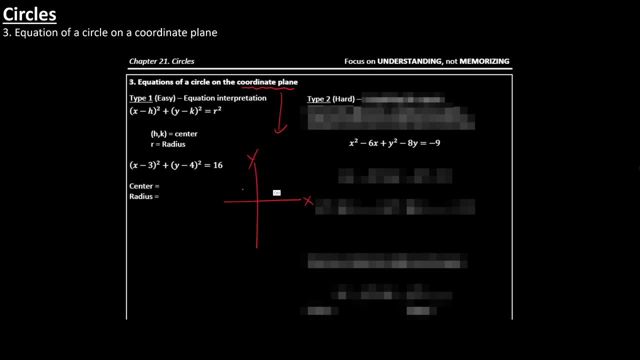 X and Y axis right, So, for instance, it might have a center right there and it might have a radius like so. but they're they're not going to give you this, They're just going to give you an equation that looks something like that, And from this you should be able to identify. 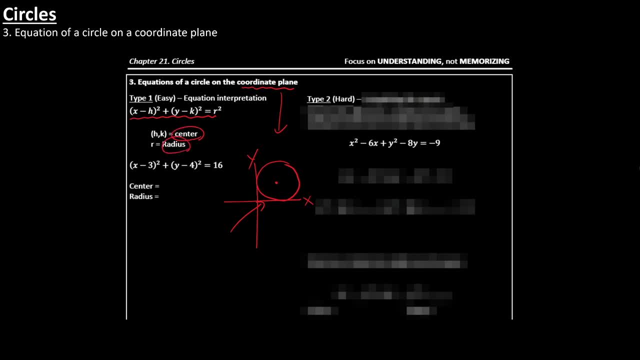 where the center is and where the radius is. That's what SAT is mainly testing you on. Okay, So you want to know the formula and how to find center and radius, And, last but not least, you also want to know what the distance formula is going to be. So for, 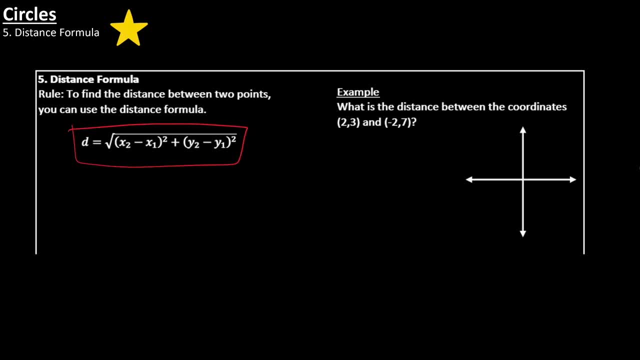 instance, distance formula is right here And the purpose of it is to find the distance between any two points, right? So, for instance, SAT might give you a question like this: What's the distance between two points? What's the distance between two points? What's the distance between two points? 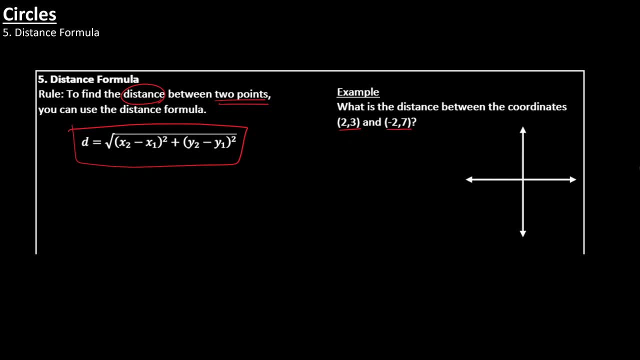 Two coordinates, two, three and minus two, seven. Well, these coordinates are going to be two, three, like right there, minus two and seven right there, And they're essentially asking you for the distance between these two points. and how you calculate the distance is by plugging it in to.